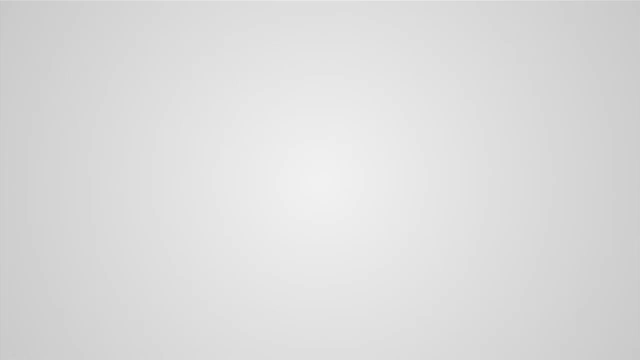 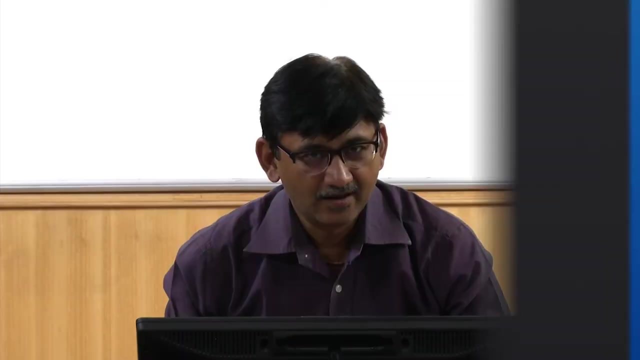 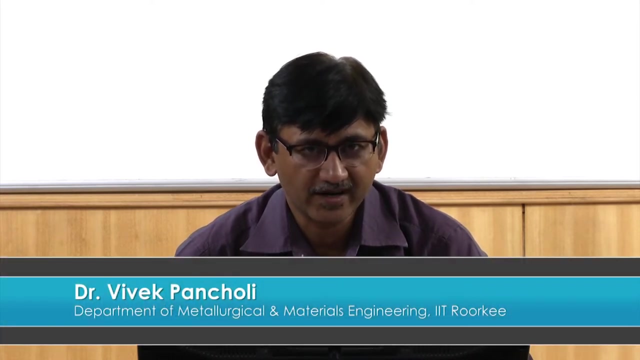 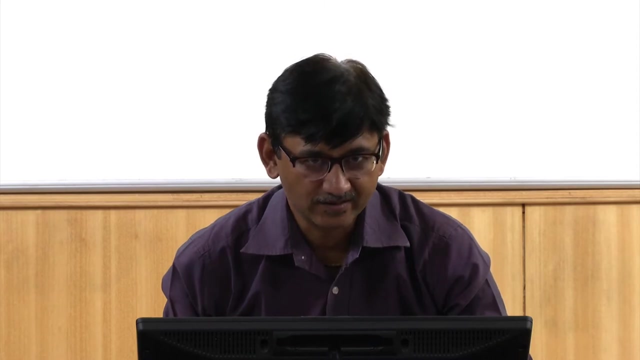 Hello friends, so till now we were discussing, I think, quite few number of lectures on phase diagram, and then we looked at some phase transformation kind of ideas and we looked at some heat treatment procedures. So now we will be shifting our course to mechanical properties, and before 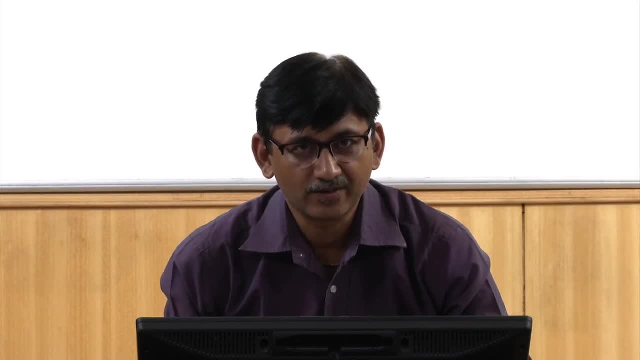 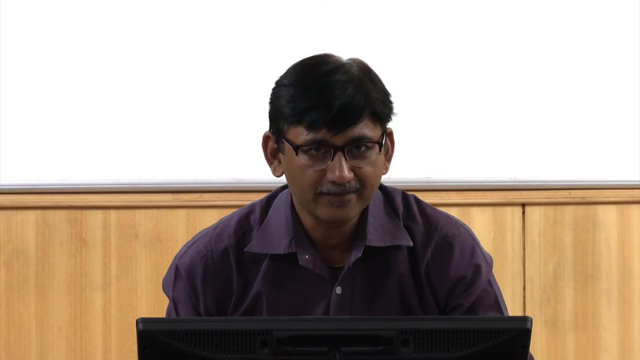 coming to mechanical properties, or what do we call as mechanical response of material to any mechanical stress or strain. So first thing we want to discuss in this is called elastic behavior. So if you look at any material, they will always show you some elastic behavior and some plastic behavior. 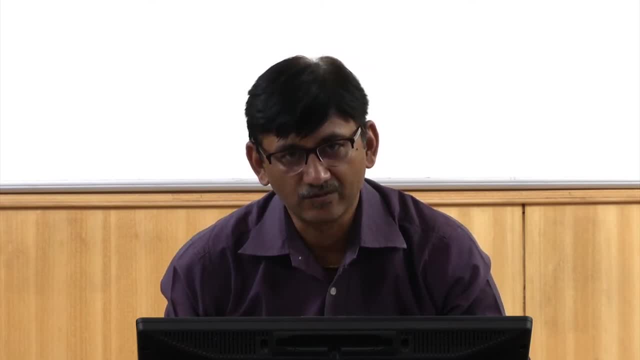 So first we will look at the elastic behavior and then we will go further and look at plastic behavior. So first we want to know that. what do we mean by elastic behavior of the material? So before that let us define few terms here. 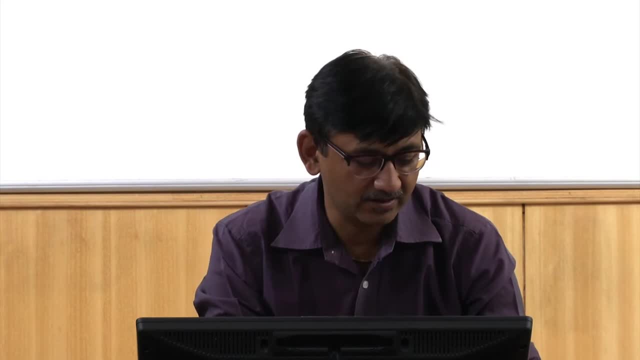 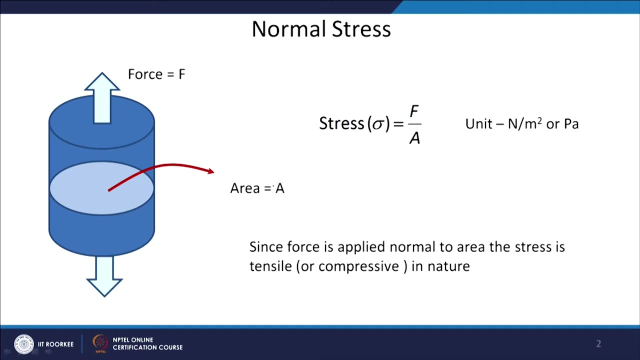 One is the normal stress. So you can see that one sample is shown here and we are showing you a cross sectional area here. So this is, you can say, cross sectional area rather than just area which is given by A, and we are applying one force here on this material. 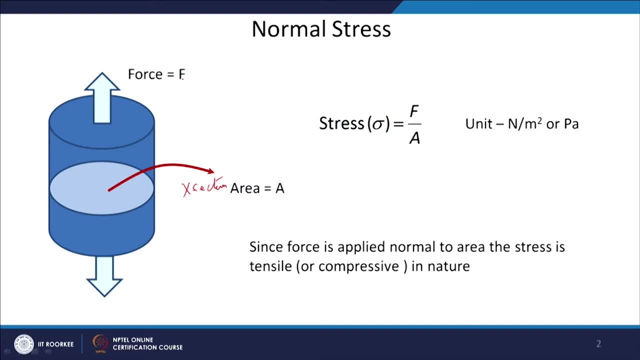 which we are saying as F. So what do we mean by stress? The stress will be defined as F, So F force divided by area, So force per unit area is the stress which is acting on this, this sample, and the unit for that will be Newton per meter square, or which is also 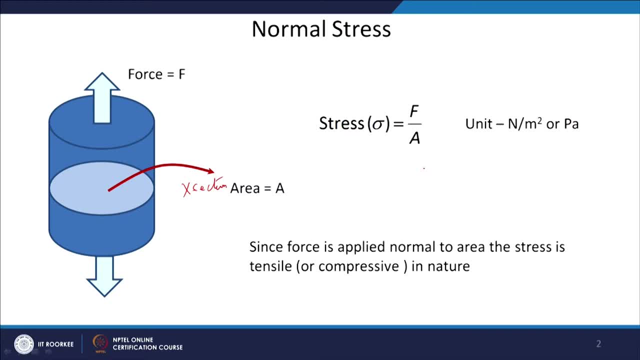 can be referred as Pascal. and since force is applied normal to the area, here the stress is called normal stress. and if this can be either tensile, So tensile means Tense, Tense, So tensile means Tense, So tensile means. 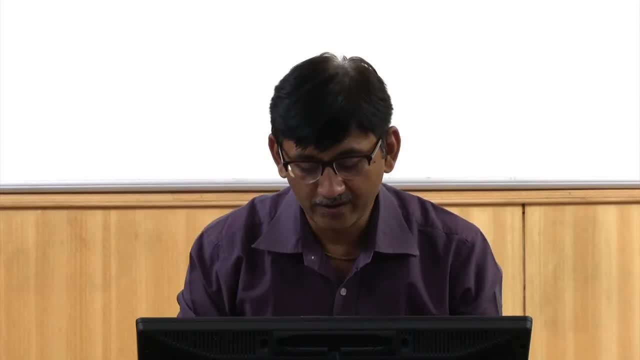 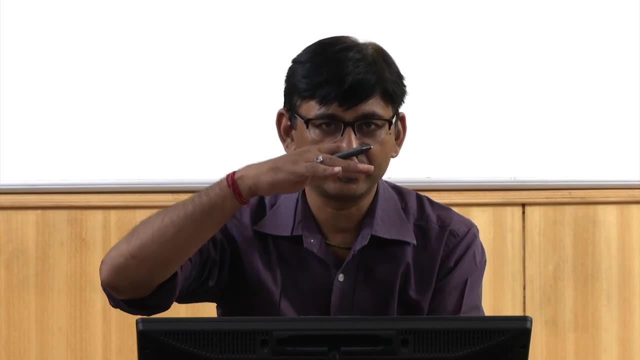 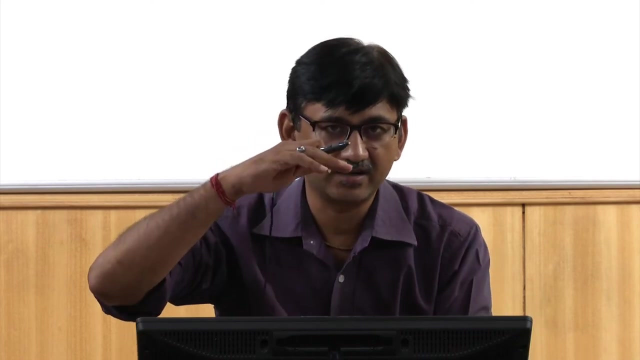 I am elongating the material or it can be compressive in nature, in which case I am basically compressing the material, or I am shortening the length of the sample, So it can be tensile where you are stretching it and it can be compressive, and in both the 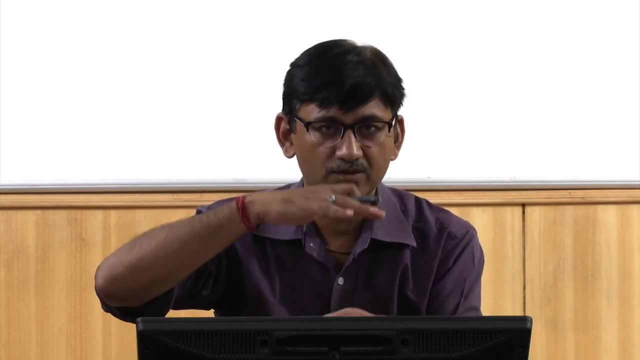 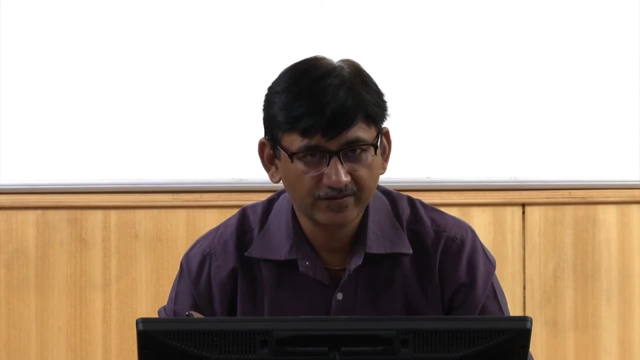 cases, because I am applying the force normal to the area, then that is why it is called normal stress. There is another kind of stress can be possible, which in which case we will call it as shear stress. So now, in this case, force is applied parallel to the area. 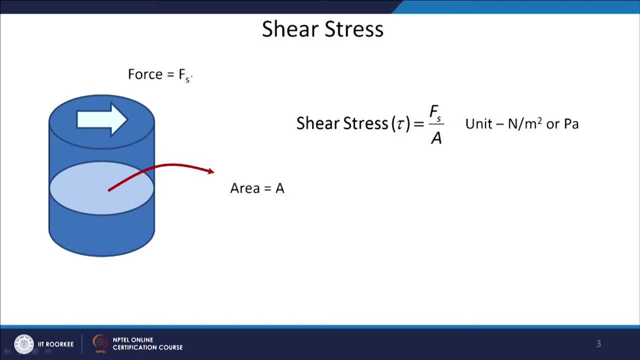 So I am calling it as Fs now because it is parallel to the area. So again, this is my area is defined and I am applying the force parallel to that. the shear stress I am defining by a symbol here is tau, which is again force per unit area. 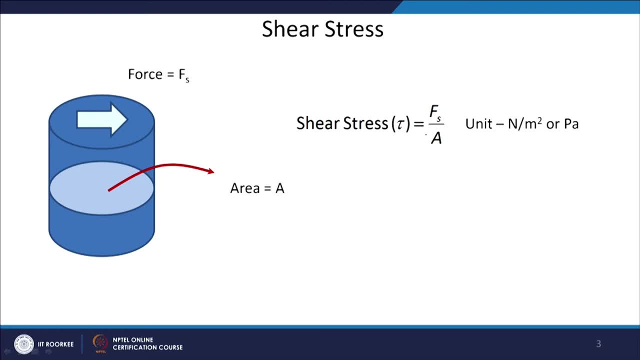 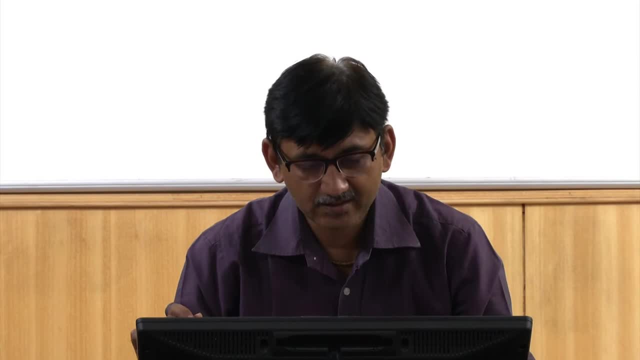 which will give you the force. So this is the shear stress. again, the units will be same as Newton per meter square or Pascal- Now there is another term. so stress can be there and similarly there can be strain. So what do we mean by strain? 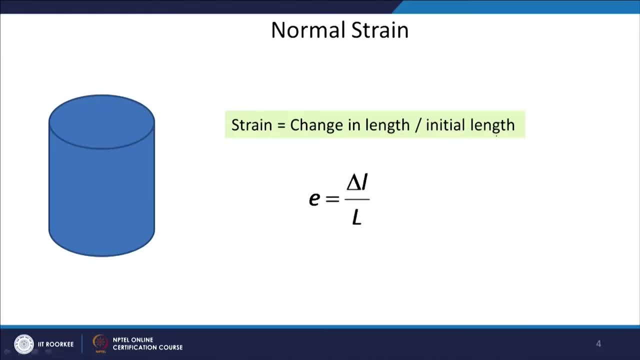 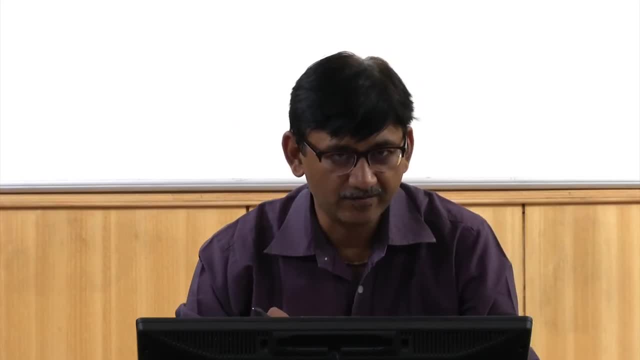 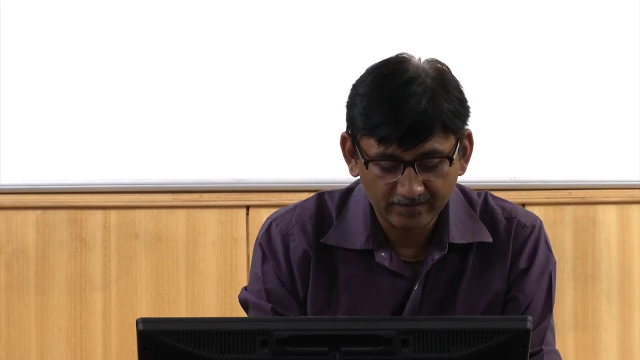 Strain is basically change in length divided by initial length. any change in the length divided by initial length is equal to strain. So basically, when you apply a force like this, I am. I have changed the length. so initial length, let us say, for my material was L and 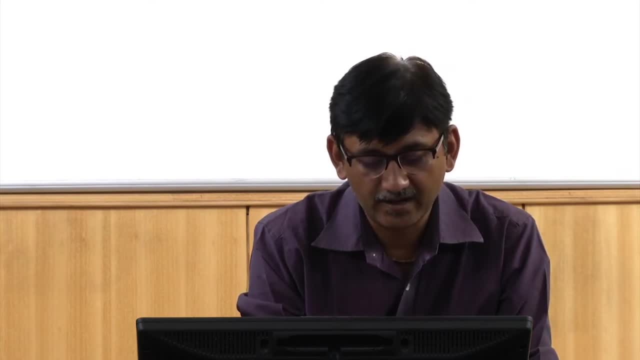 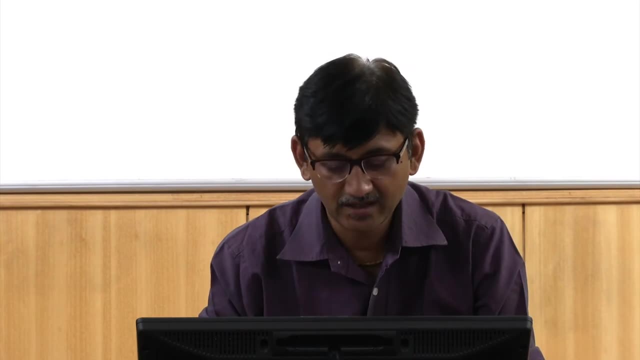 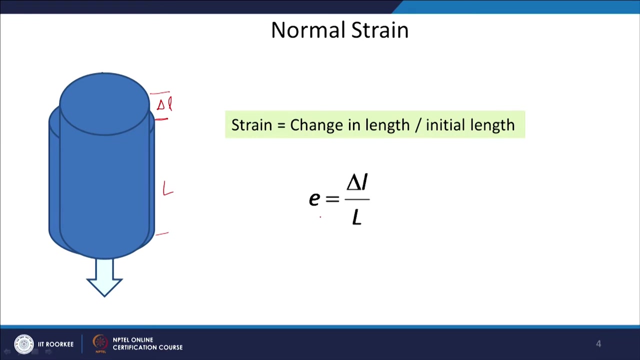 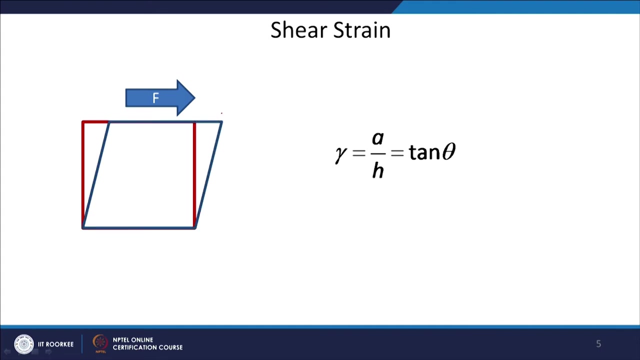 the change in length is, let us say, given by delta L, then the strain will be change in length, which is delta L divided by the initial length. that will be equal to the normal strain, again, because I am measuring the strain. So this is the strain from the fixed end, which is H, A by H, and that will be obviously. 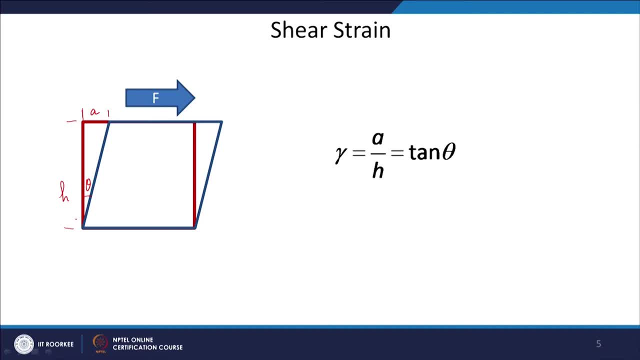 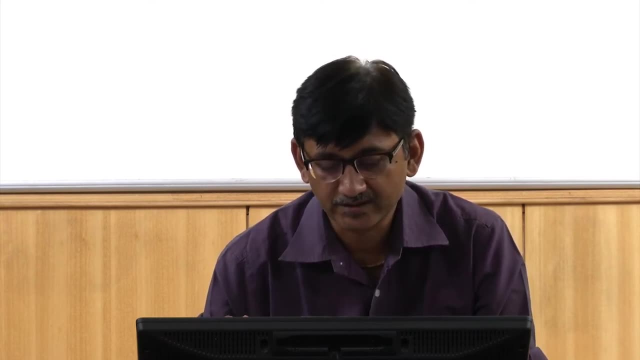 because this is a perpendicular and this is the base. perpendicular upon base, then, and this is angle theta, So it will be equal to 10 theta. So this is the shear strain, because of the shear stress on the material, whatever strain is produced is called shear strain, and that will be equal to A by H, equal to 10 theta. 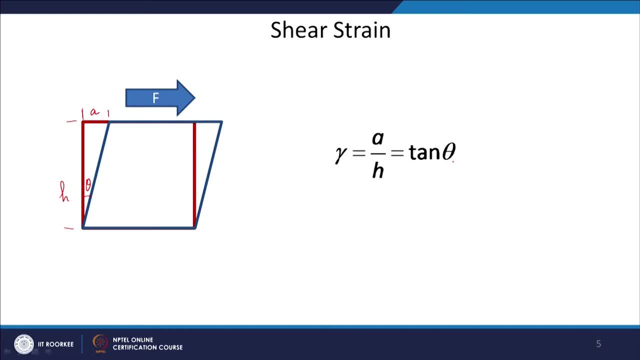 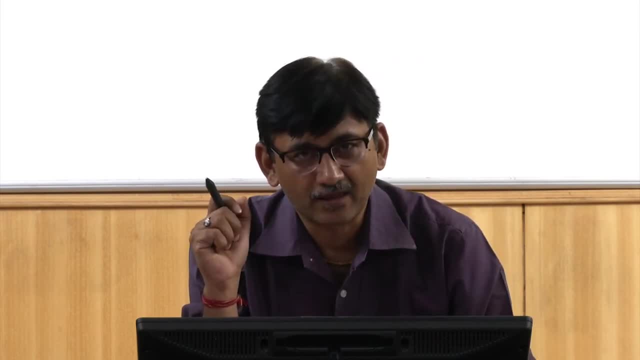 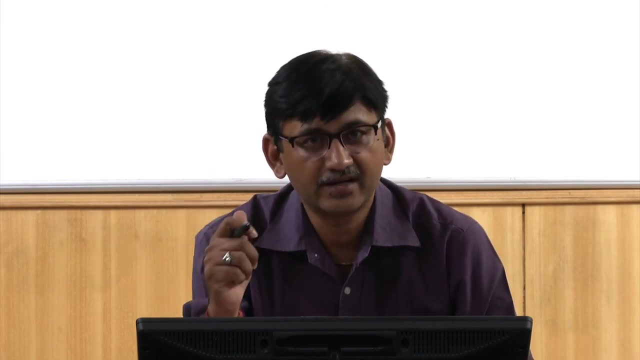 So this is the definition for stress and definition for strain. very quick definitions. we are doing here for a very detailed definition of stress. I would suggest that, as a mechanical engineer student, you must be going through a course called strength of materials, In that you will see a detailed definition of stress. we are not doing it here for that. 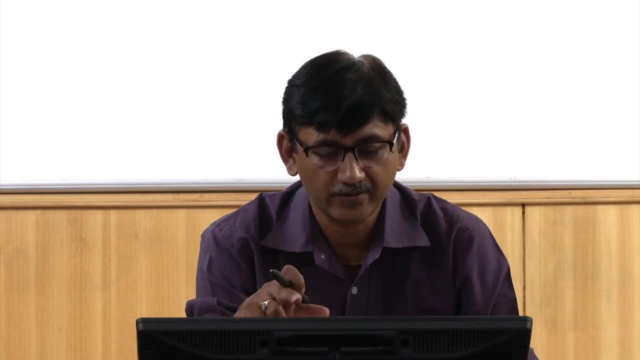 how is to go through that particular course? Now, what is elastic behavior? So once we have defined stress and strain, now we can look at elastic behaviour of the material. it is the material. if material recovers its dimension after removal of load. 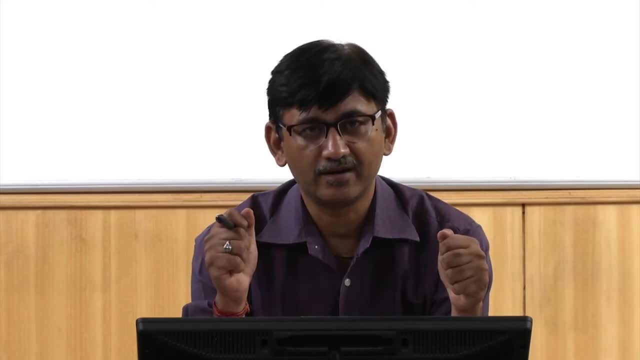 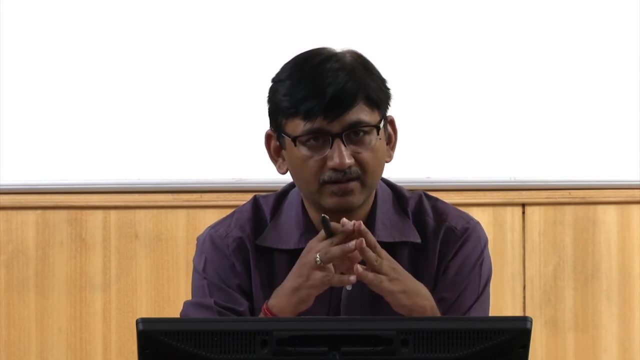 So if I have applied a load and when I remove the load it goes back to its original position. good example of understanding this type of behavior is: you can see in springs. ok, So you take a spring, you compress it and when you leave the load it will go back to its. 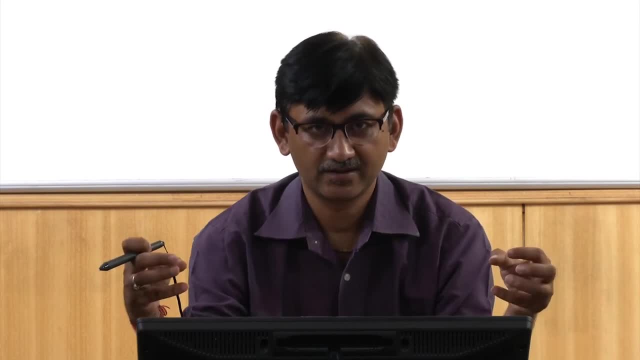 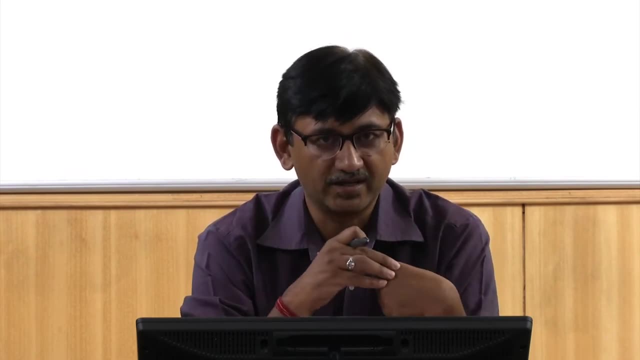 original position. ok, for if I stretch it, ok, and when I remove the load, it will again go back to its original position, ok. So spring is one example very, very close to this idea. of course there are no. there is no spring when we are talking about material, ok, but 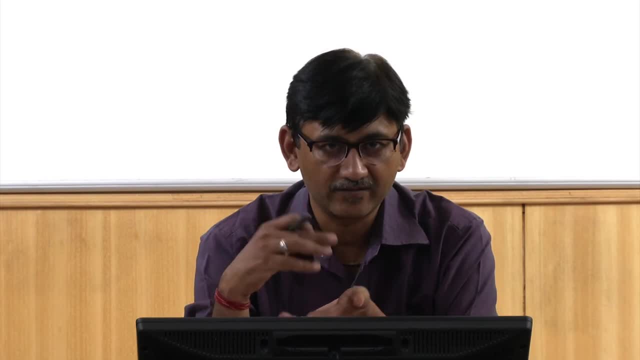 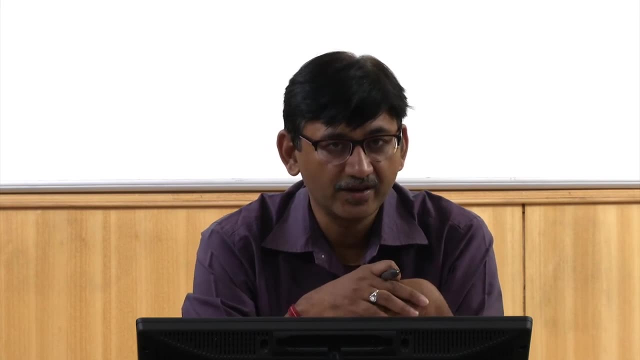 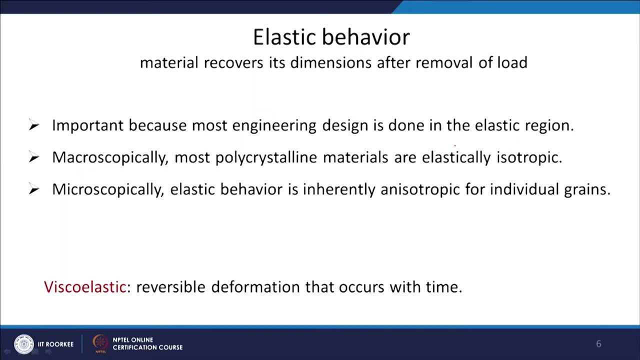 the behavior is same that when I apply the load, ok, it will deform. when I remove the load, it will come back to its original position. Why we are understanding of elastic behavior is important. It is important because most engineering design is done in the elastic region. as a mechanical engineer, whatever design, 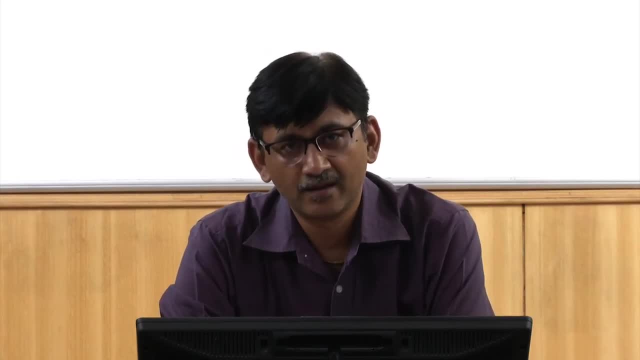 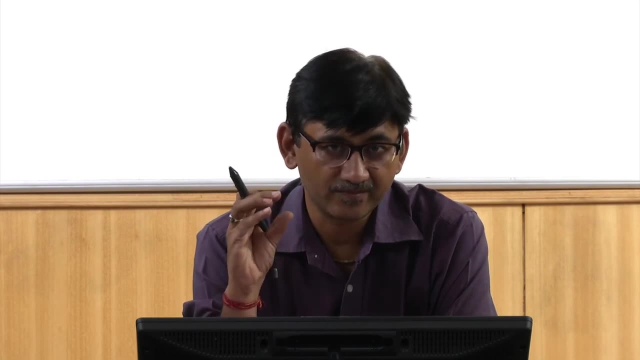 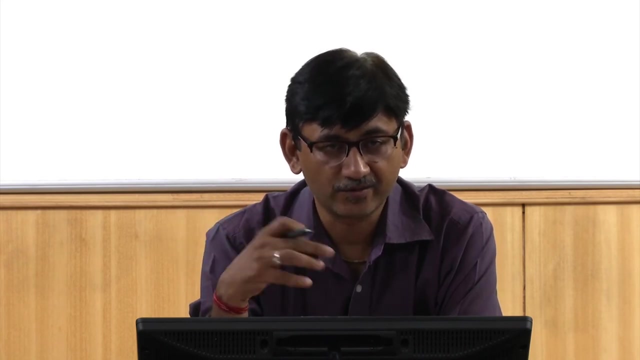 you are going to do for any structure. ok, It has to be done under elastics, Elastic limit. ok, that means it has to be done where the material show elastic behavior. You cannot cross the yield or you cannot cross the limit where it starts deforming plastically. 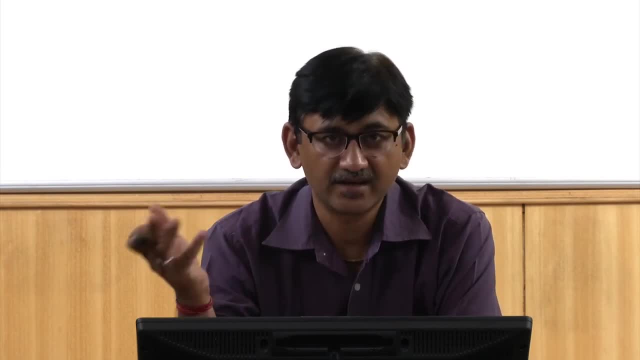 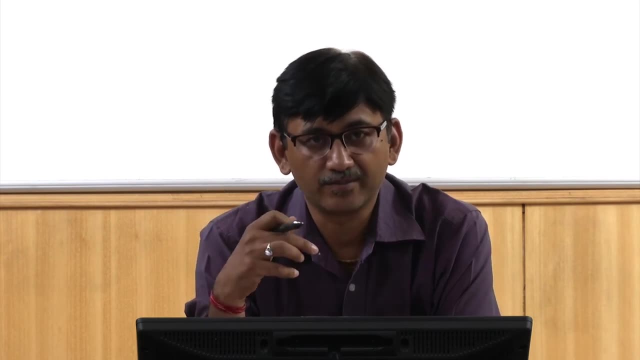 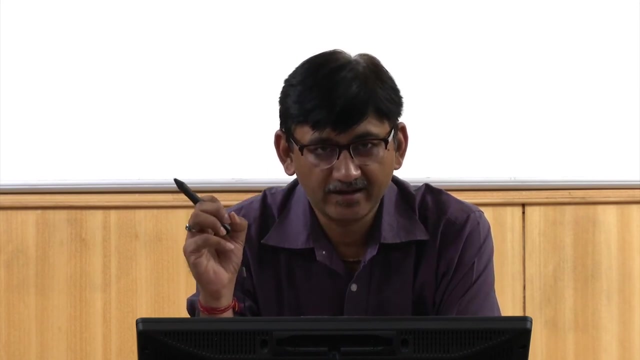 ok, Because if it does deform plastically that means it the material is failed. ok, So in the strength of material approach, again that that will come to understand as a yield or material criteria. So for any engineering design it is important that your material 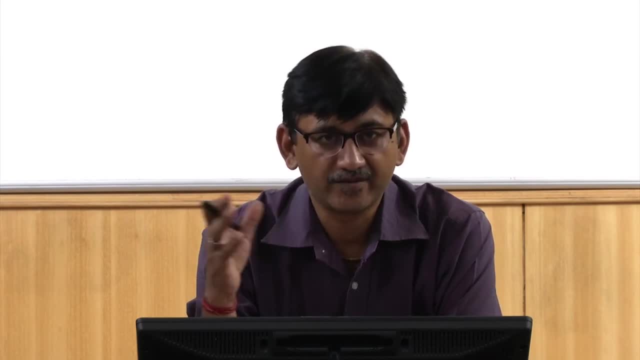 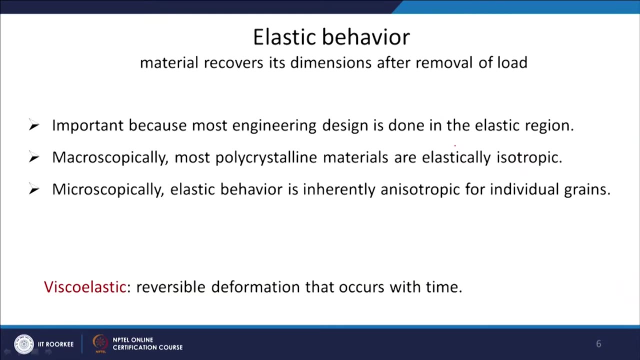 should not cross the elastic behavior of region. ok, Microscopically, if you see, most polycrystalline material are elastically isotropic, So we do not have any problem of that. they may show anisotropy. microscopically it can have anisotropy. 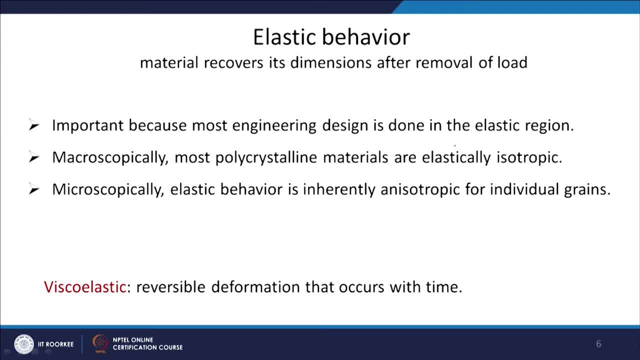 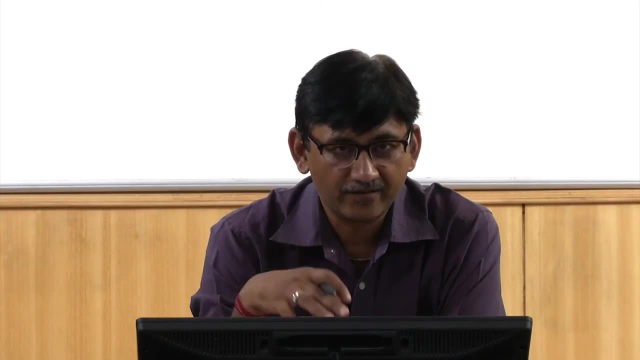 but since materials- most of the engineering material- are polycrystalline, I do not have to worry about that. then there is another concept called viscoelastic properties of material, in which case this reversible deformation that occurs is dependent on time. if it is not a viscoelastic, normal elastic behavior, then as soon as I leave the load it will go. 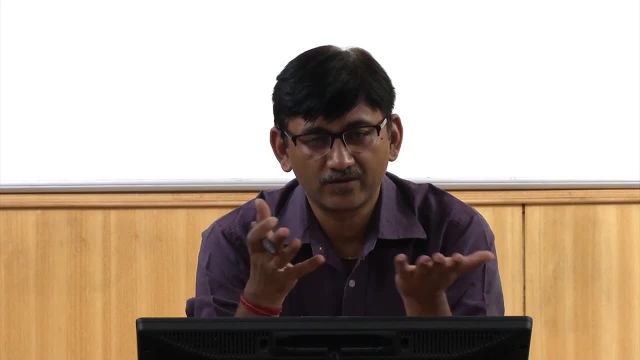 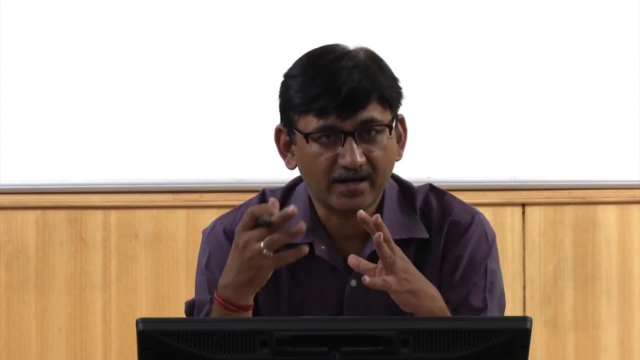 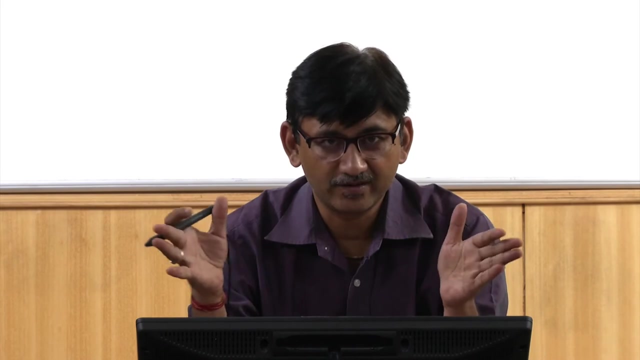 back to its original position without any time delay. but if there is any time delay involved in this, and as I told you earlier also that any time factor when it comes it is called visco is a prefix is added. so if the reversible deformation is time dependent, 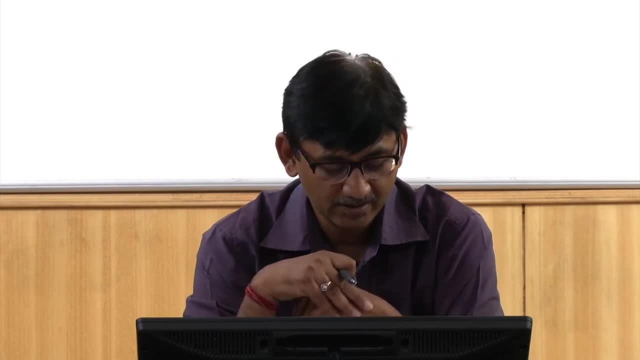 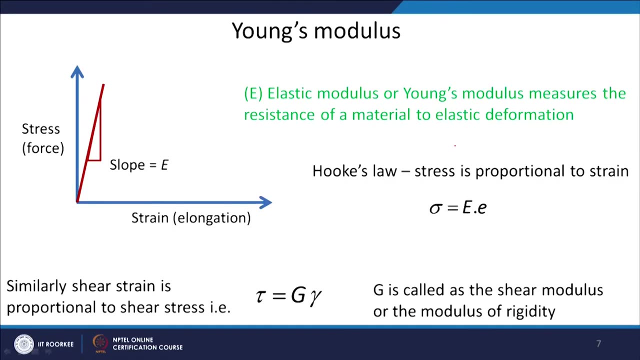 it takes some time to go back to its original position. then that is called viscoelastic behavior. So this is how elastic behavior will look like in a typical stress strain curve. so you have stress on the y axis and strain on the y axis. Please remember, when we show something like this, we are showing it in, because when we 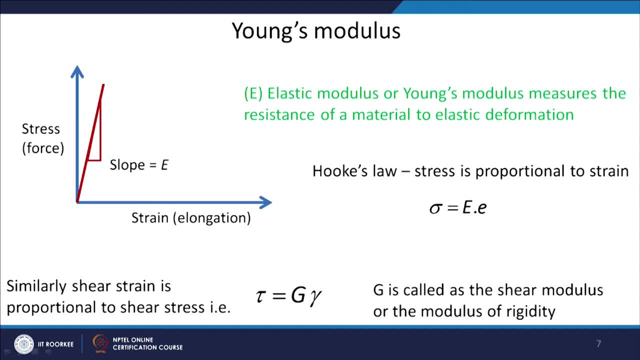 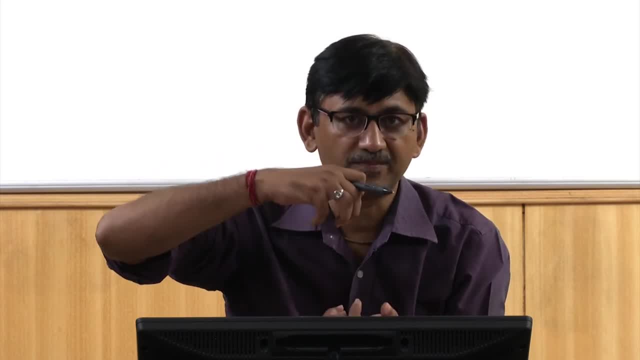 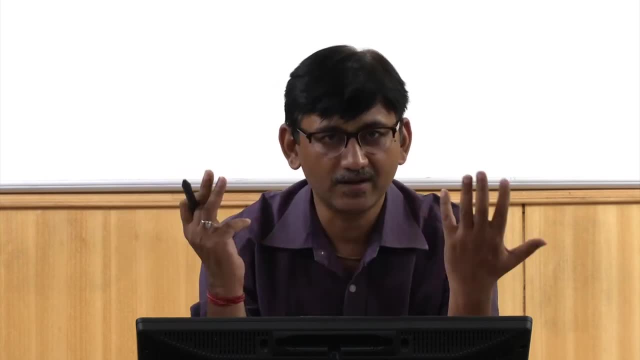 do a tensile test. what we impose on the material is the strain, not the stress. we force the material to deform and the stress is the response of the material to this elongation or strain In normal practice. basically, we apply the load and the material response is in form. 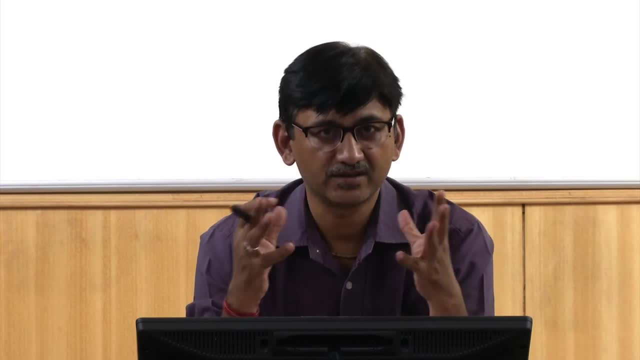 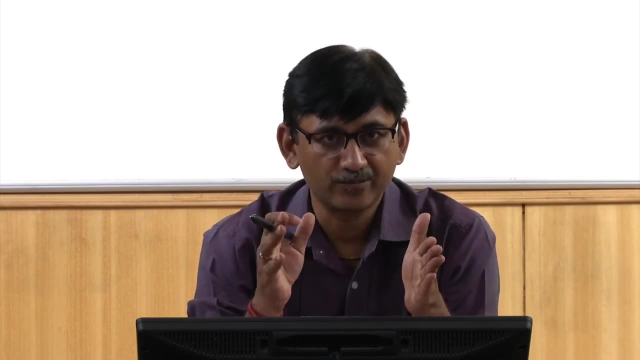 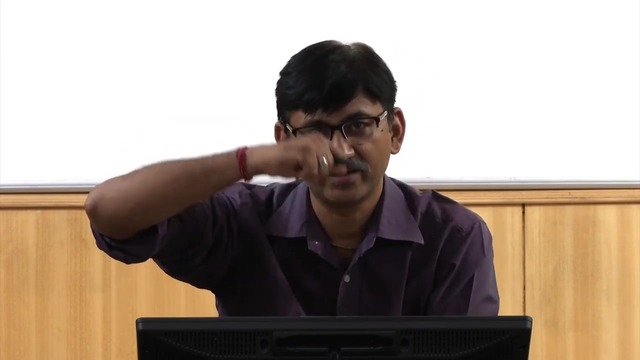 of stress. So there can be different situation in different cases. but when we do a tensile test, what we are imposing, or what is the independent variable, is strain. I am deforming my cross head of the machine is moving and it is deforming the material. it is imposing a strain and material. 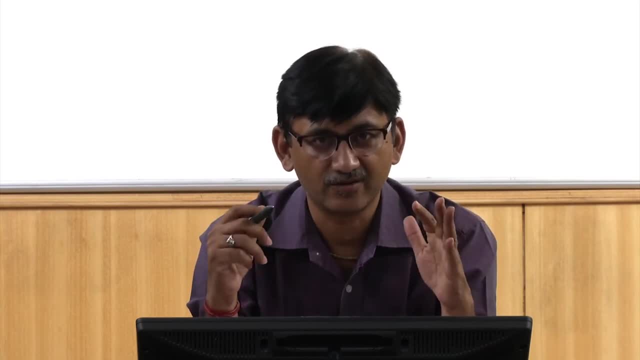 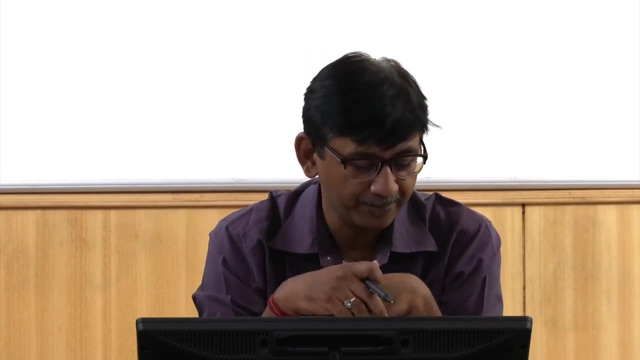 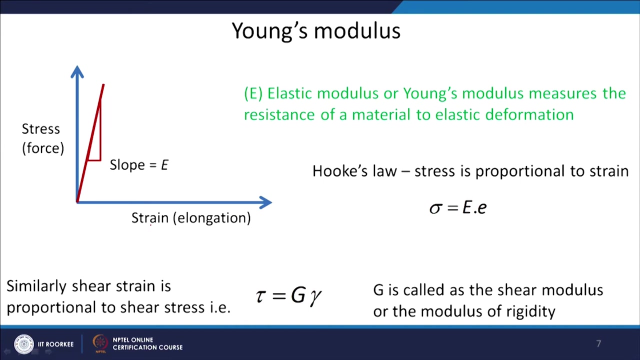 is responding in form of stress and that is what is measured using load cell in the machine and that is what is reported. So basically, on the x axis it can be elongation, movement of the cross head or you can convert that into strain because delta l by l, it will also give you force from the machine. that 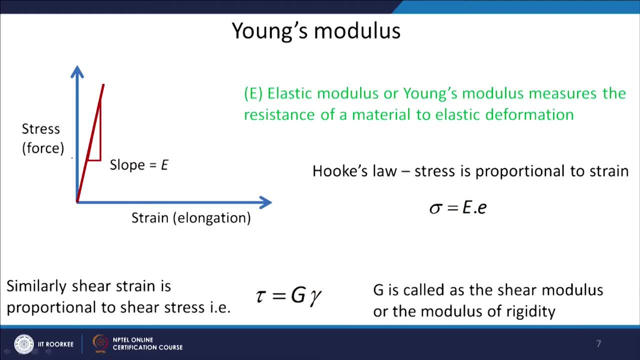 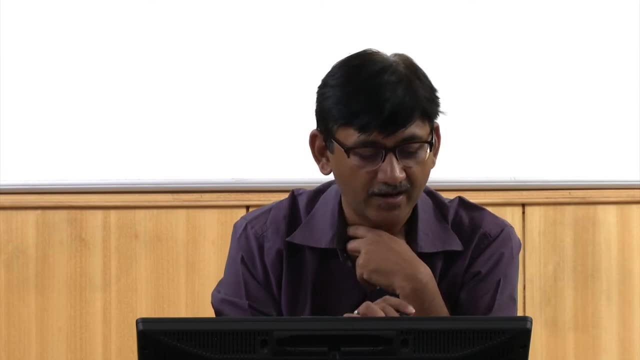 can be converted to stress. so force divided by initial area, that will give stress and the elastic in the elastic part it will have this linear behavior between the stress and stress, in strain and stress. So stress is linearly dependent on strain and the slope of this. 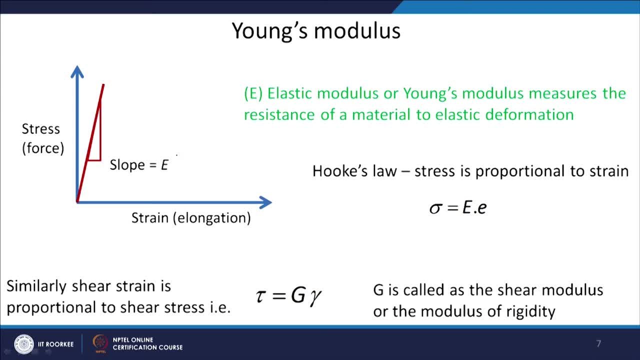 linear curve is what we call as elastic modulus or Young's modulus, E. So slope of the curve will give you E and this linear independence of stress on strain, which is what we call as Hooke's law. stress is proportional to strain, So sigma is equal to E into strain. 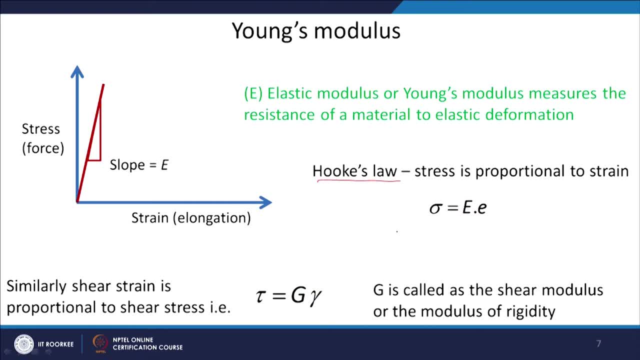 that is what is Hooke's law, What it measures. the elastic modulus, or Young's modulus, measures the resistance of a material to its elastic deformation, as I told you that, whatever deformation, I am imposing its resistance. So if you have high elastic modulus, that means resistance. 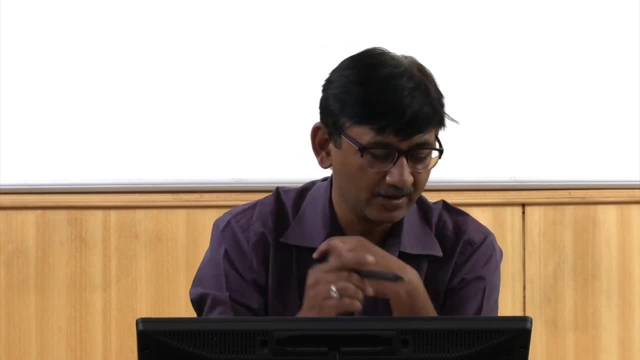 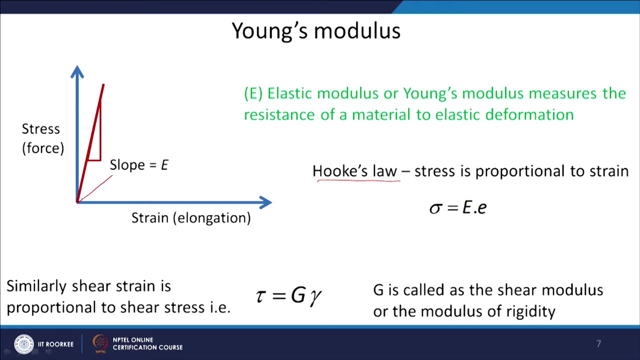 will be more. it will. you will really require more stress. So if a material has low elastic modulus, the it will be slope will be small. if material has very high elastic modulus, the slope will be high, So resistance will be high for the same amount of deformation. in this case the stress is 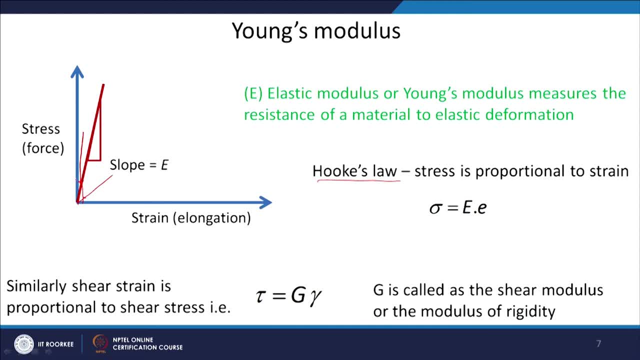 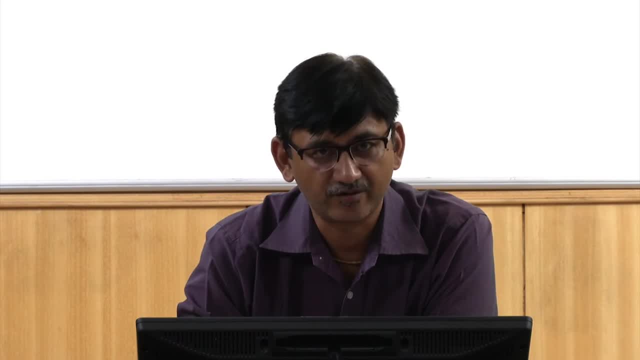 this much. in this case, the stress is this much. resistance has increased. So it gives you a resistance to deformation and it is the response of the material in form of a stress when you are imposing strain. in case of shear strain also, you can do same. 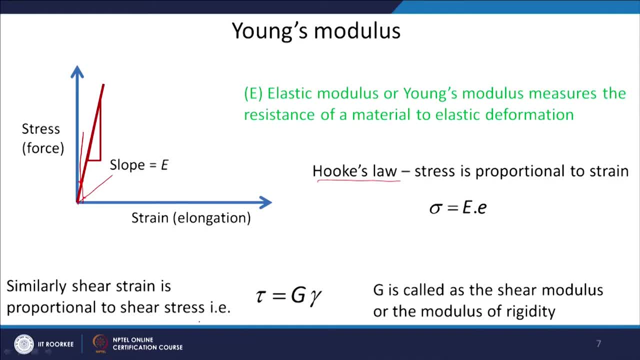 thing. similarly, shear strain is proportional to shear stress. so sorry, shear stress is proportional to shear strain. So I will just do some small correction here, so that tau is equal to g gamma. So here you are getting a new elastic modulus, a new elastic constant, which is the shear. 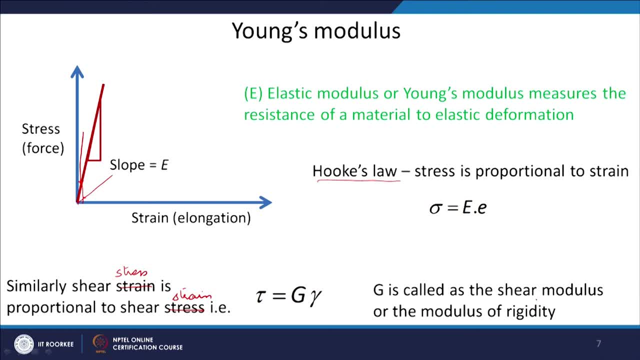 modulus or modulus of rigidity. So when I am doing under shear condition, then I am going to use the shear modulus. when I am doing in a tensile, uniaxial tensile or compressive type of experiment, then I will be relating the stress with a strain using Young's modulus. 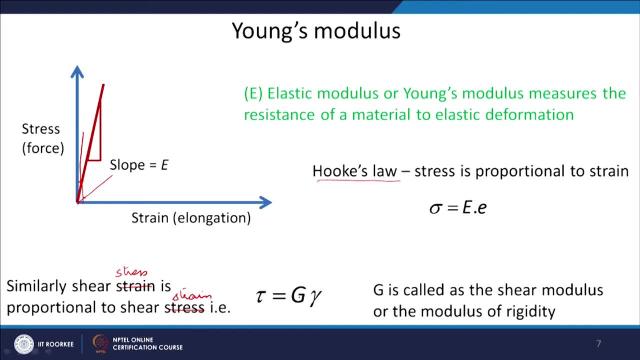 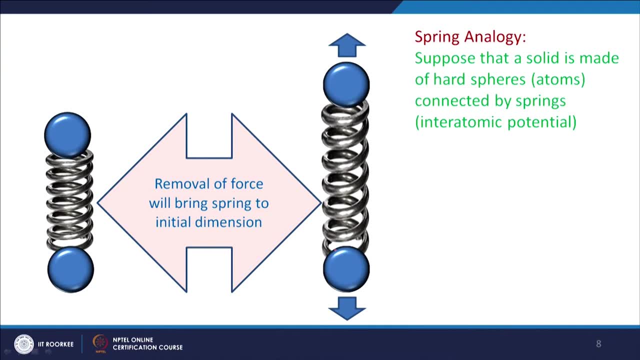 So what type of deformation I am doing? I have to choose elastic constant accordingly. So this is the spring analogy for elastic deformation, as I told you. Okay, So you have atoms, and atoms are basically having bonds between them, and then bonds can. 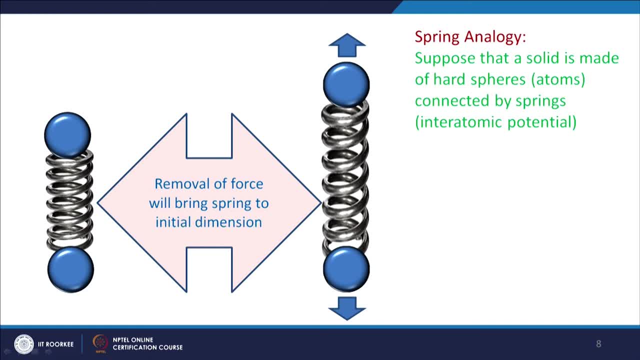 be considered as spring. So when I am deforming it the spring is getting stretched. So as soon as I remove the force it will go back to its original position. So removal of force will bring spring to initial dimension. So I can use a spring analogy to explain this: that solid is made of hard sphere, which 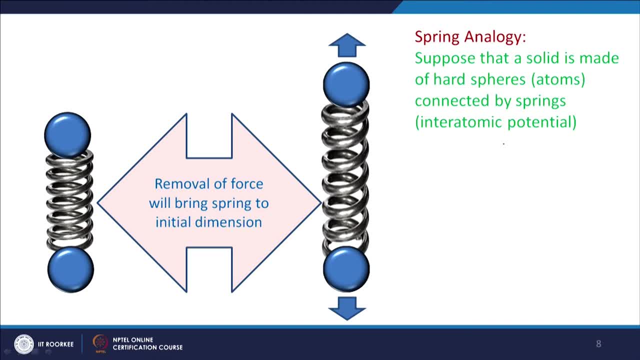 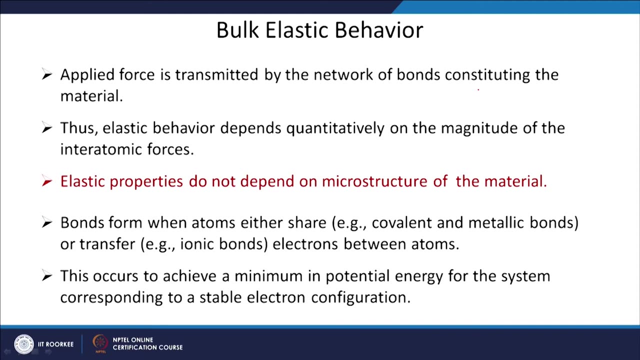 is an atom and connected by spring, which are inter atomic forces or potential, And as soon as I remove the force, it will go back to its original position. So basically, if you look at elastic behavior, applied force is transmitted by the network of bonds constituting the material. 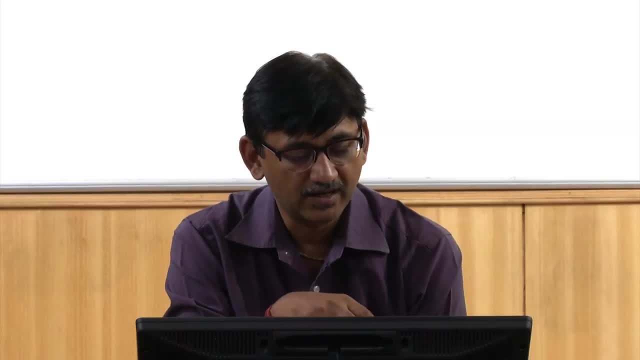 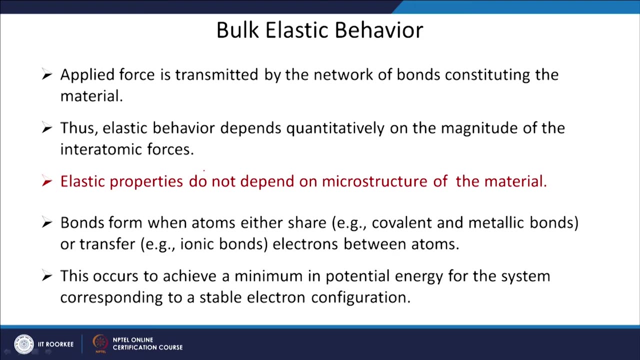 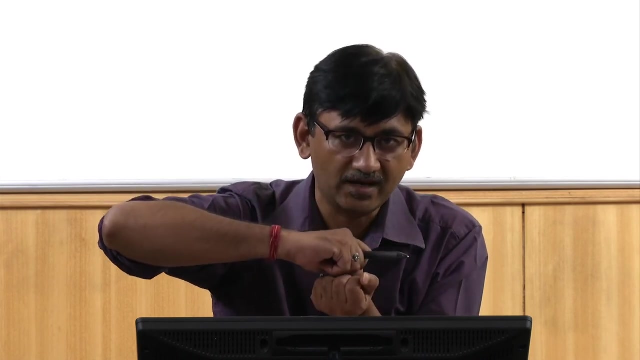 So of course there are bonds between the atoms. the elastic behavior depends quantitatively on the magnitude of the inter atomic forces. So if you have a stronger bond- Yes, Yes- Then you will require more force to deform it. That means the elastic Young's modulus of that material will be high. 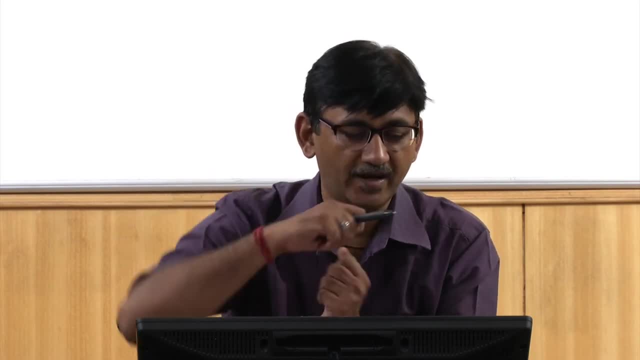 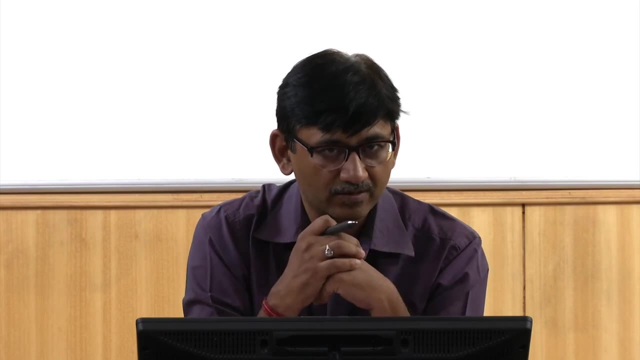 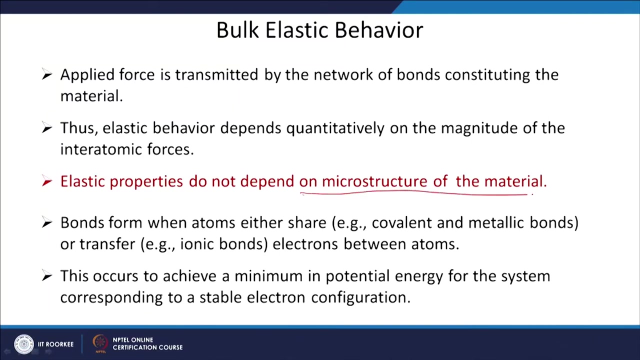 So if stronger bonds are there, elastic modulus will be high. Young's modulus will be high. More inter atomic forces, you have more bond strength, more Young's modulus. Elastic properties do not depend on microstructure of the material. this is very important to note that my Young's modulus 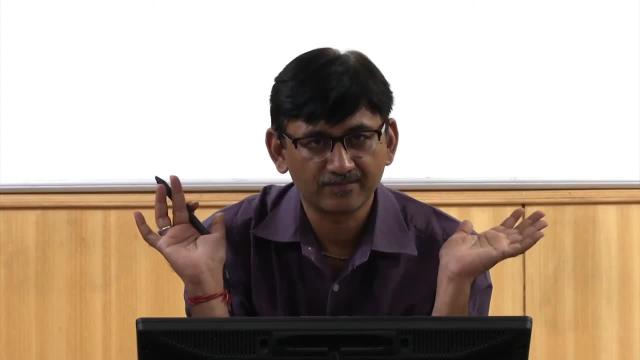 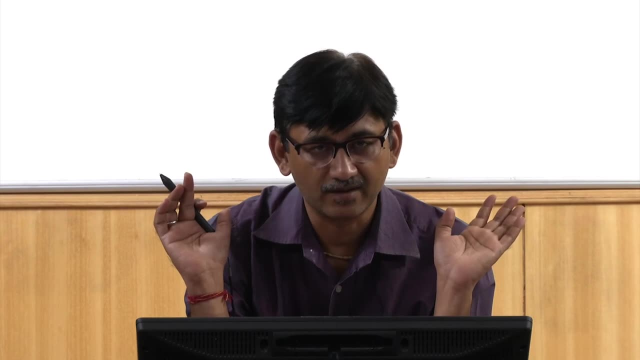 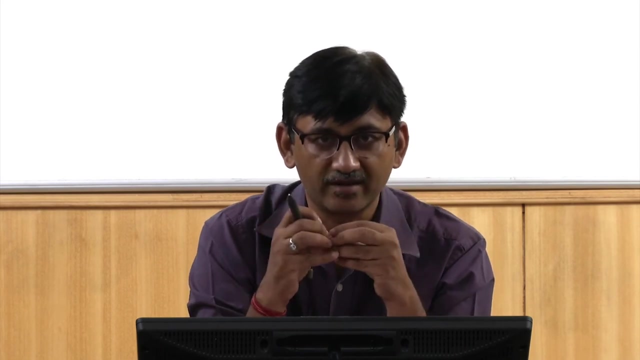 Yes, It does not depend on the microstructure of the material. So you can have fine grain, you can have coarse grain, whatever it is not going to depend on the on the microstructure, the elastic modulus. It is only dependent on the bond strength and that is not changing. 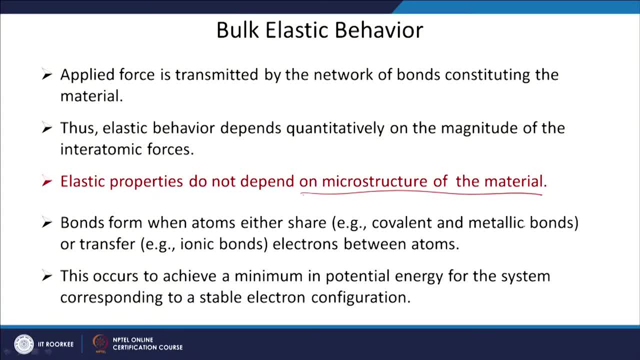 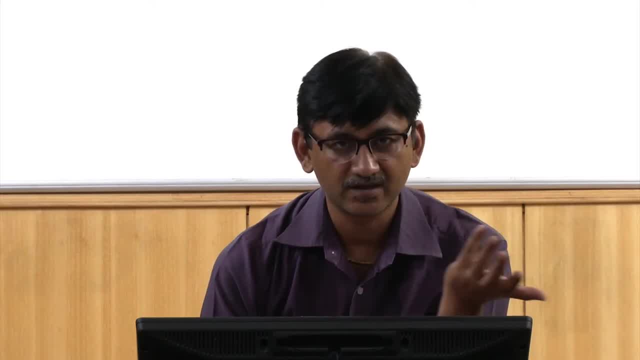 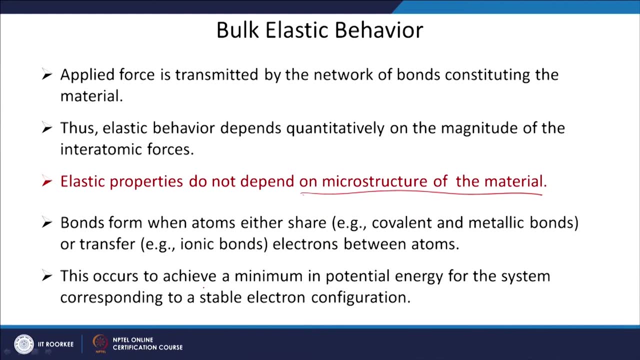 So bond force, an atom, either shear- example, it can be covalent, or metallic bonds, or it can be ionic bonds. So depending upon different type of bonds, you will have different bond strength and different elastic modulus. Of course the bond strength, bond length should be such that that it is minimizing the potential. 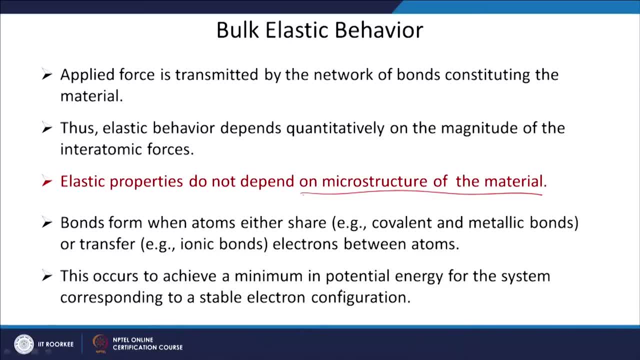 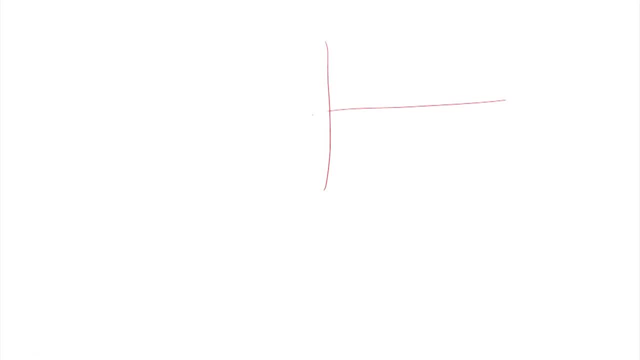 energy for the system. So let me just bring this aspect out. If you see, in terms of potential energy, the curve for potential energy is something like this: Ok, This is the distance, so it will be something like this. this is the position where you 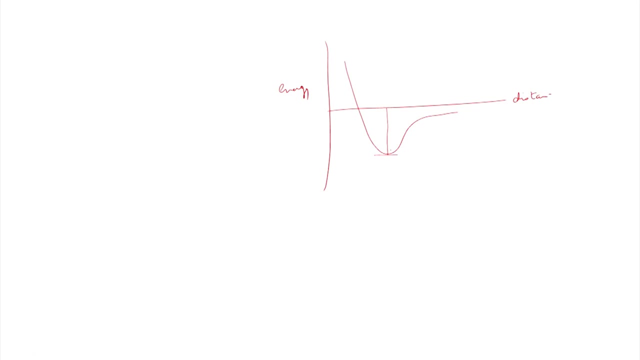 will, are going to have minimum energy. So this is, this will be the bond length. so distance between atoms. So this is the distance. Yes, Ok, Yes, So this is the distance, equilibrium distance. If I bring them closer, the potential energy will increase. if I then take them apart again, 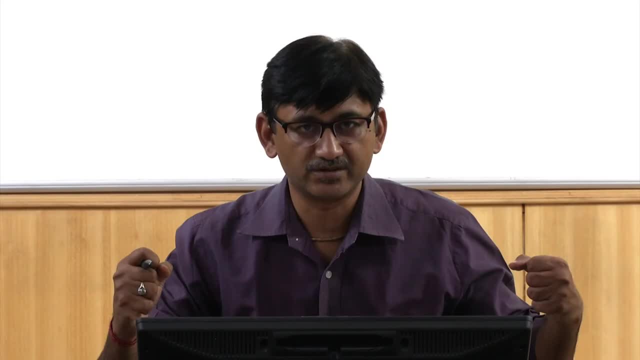 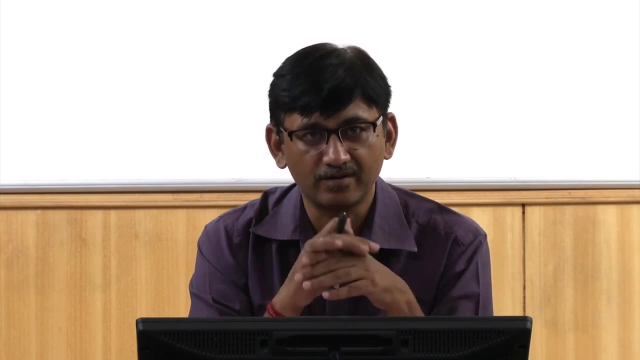 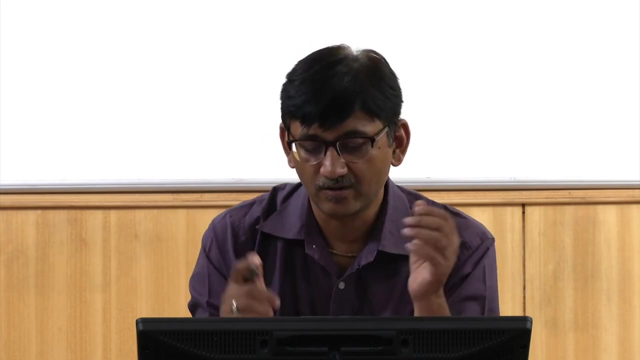 the potential energy will increase. So whether I do stretching or whether I bring them closer, in both the cases the potential energy will increase, and that is what we do not want, and that is what atoms do not want. So as soon as I remove the force, it will try to go back to its minimum potential energy. 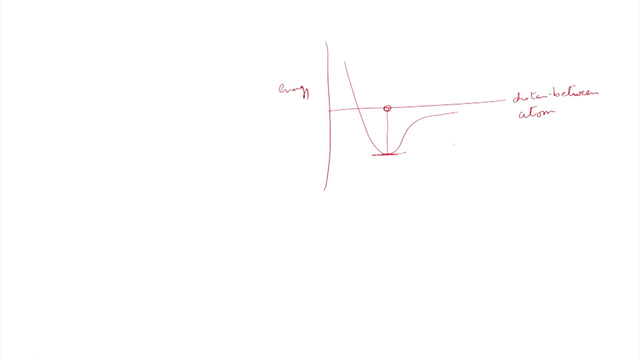 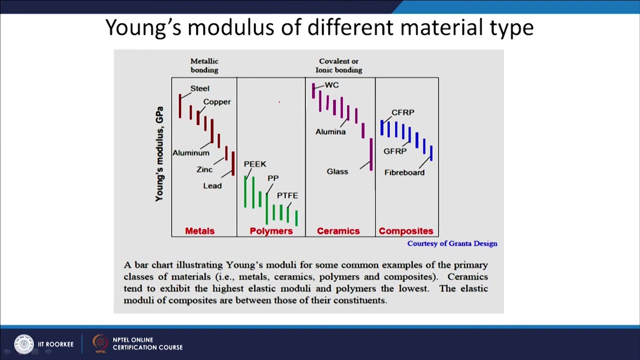 configuration, which is what is the equilibrium distance between the atoms. So this is what is the driving force for elastic deformation. These are some values of Young's modulus of different material type. So you can see that covalent or ionic bonds are very strong bonds. 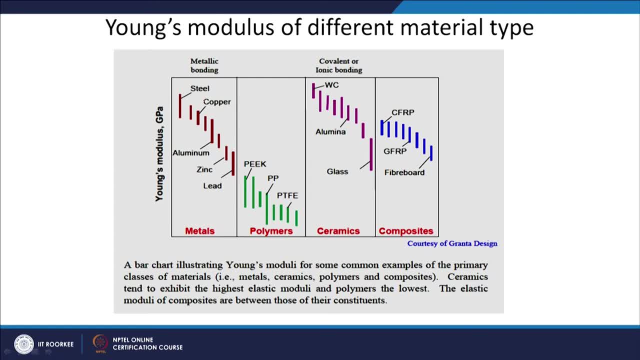 So very high elastic modulus and this is for metallic bonds. steel has very high long elastic modulus, So these are very high elastic modulus than copper, aluminium, zinc. depending upon their bond strength They will be grouped in different categories here. Some for polymers also are shown here: polymer and composite. 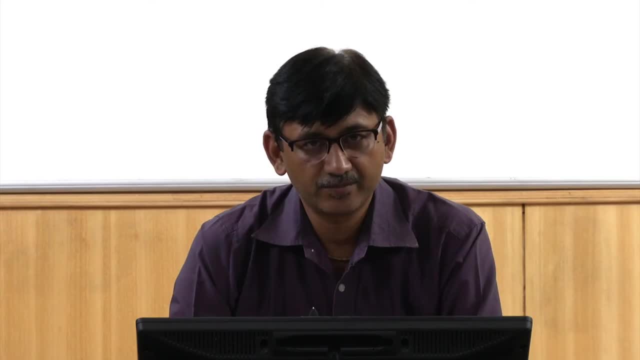 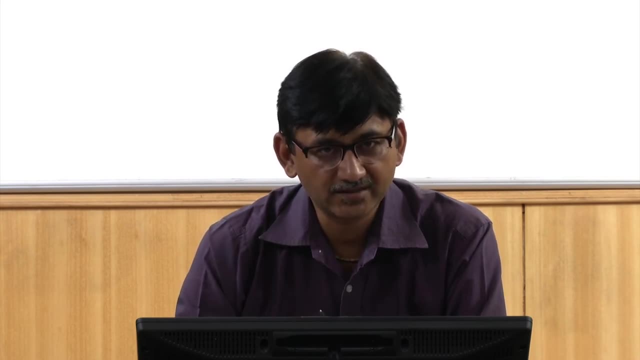 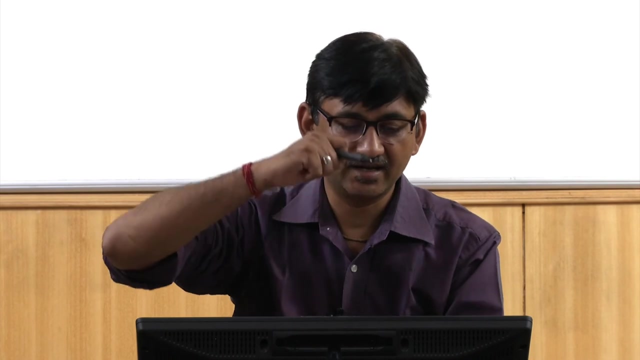 Now, after understanding the elastic deformation and Young's modulus, there is another very important parameter when you are doing deformation under elastic limit is called Poisson's ratio. What does it mean? That when I am applying a tensile stress, for example in z axis, in this direction, so when 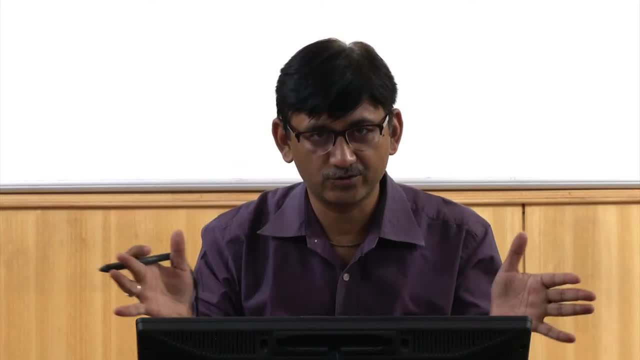 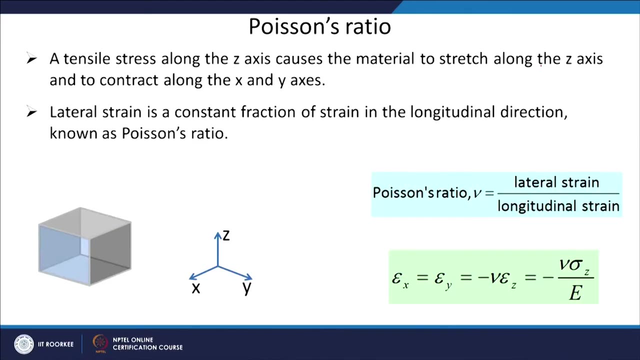 I am elongating in z axis, z direction, there has to be contraction in the x and y direction. So that is what is there. So when I am doing a stretching along z axis, there has to be contraction along the x and y axis. 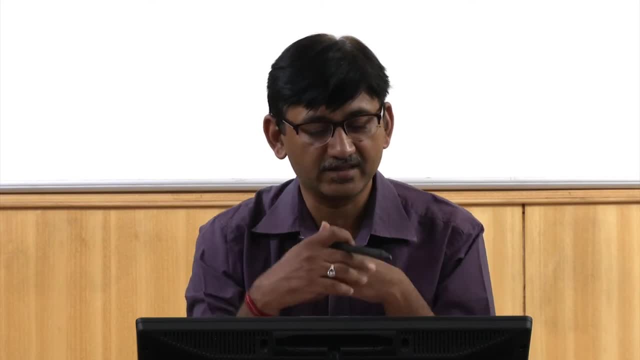 The lateral strain. lateral means this: two in x and y direction is a constant force. So this is the tension, So this is the tension, So this is the tension, So this is the contraction of a strain in the longitudinal direction, that is, the in. 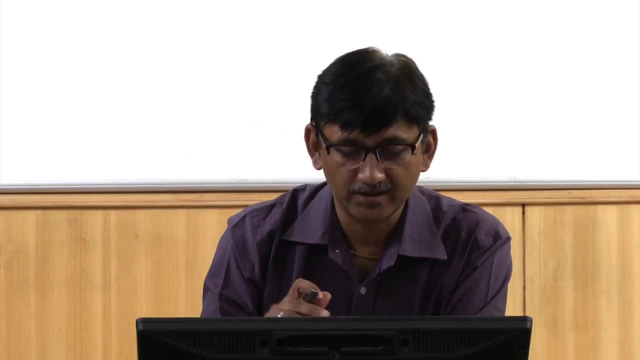 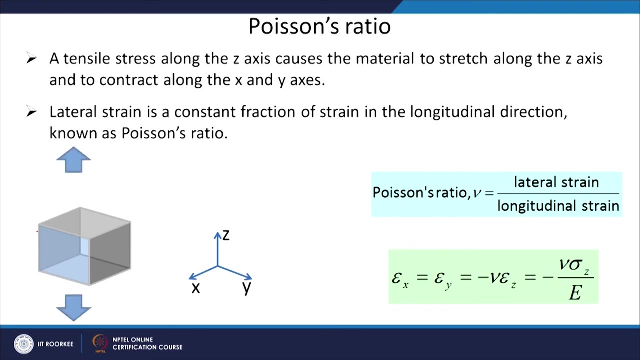 the z direction and that is known as Poisson's ratio. So suppose this is a cube as shown here, and I want to apply a force here in z axis and because of that it will deform, elongate in z direction and there will be contraction. 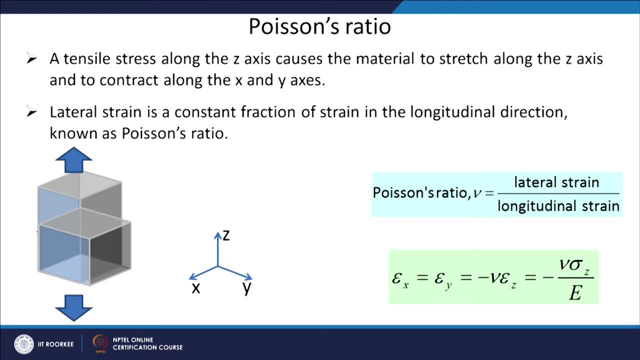 in x and y direction. So if you measure all these dimensions, So the strain in the x or y direction divided by the strain in the z direction will give you the Poisson's ratio. So Poisson's ratio nu is equal to lateral strain. about longitudinal strain. 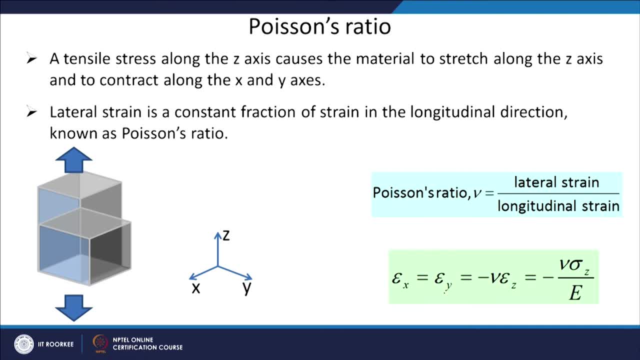 So epsilon x in the x direction or epsilon y in the y direction is equal to minus nu of epsilon z. Why we are keeping minus sign here is because if a strain in the z direction is tensile, the strain in x and y direction is: there is a contraction, there is a negative dilation. 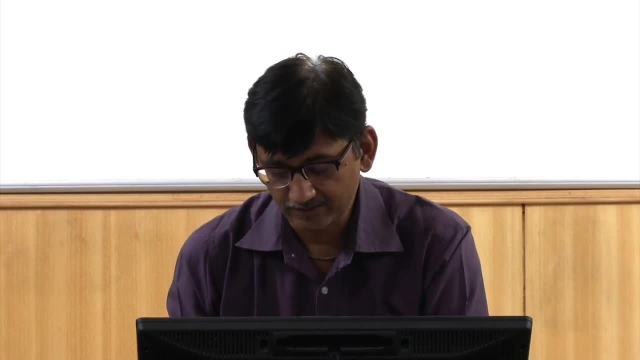 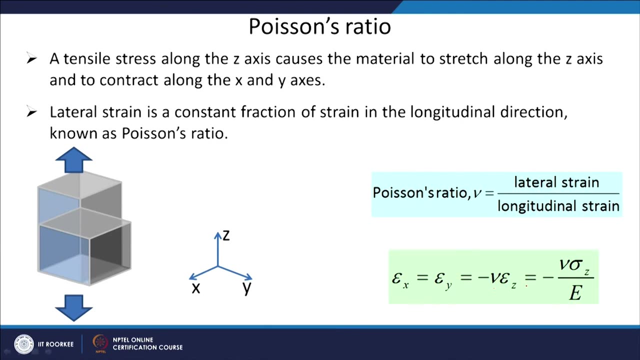 So that is why we are using minus here, that epsilon x will be equal to minus of nu into epsilon z, or epsilon y is equal to minus of nu into epsilon z. So if one is tensile, other way has to be compressive, and that is why the negative sign. 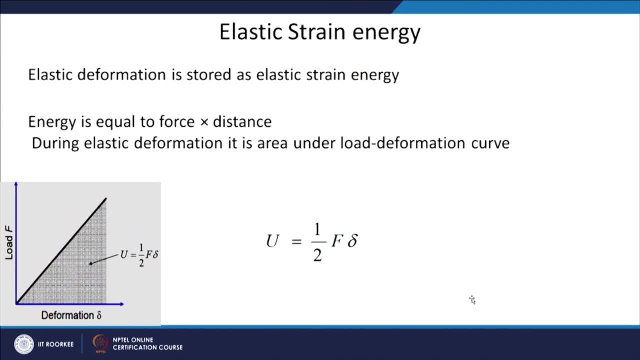 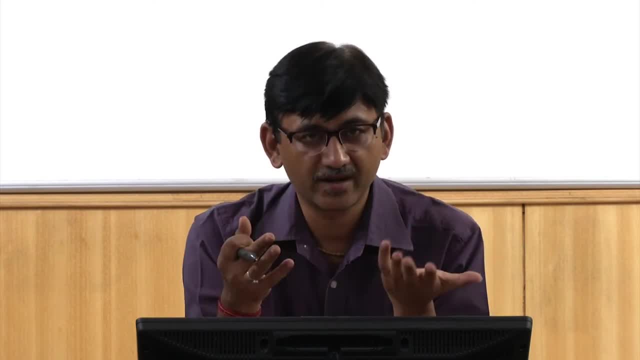 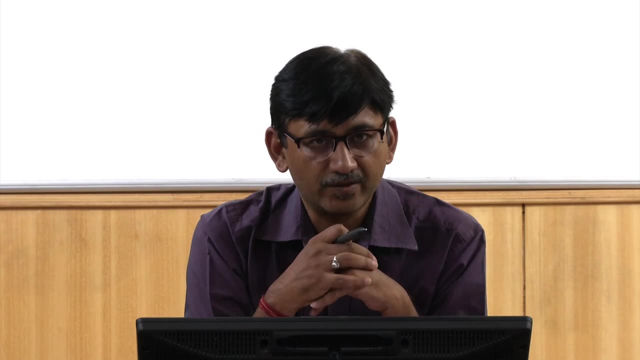 Now there is another concept called elastic strain. energy is, as you can see, that when I am deforming it, my potential energy is increasing. that means I am storing the strain energy in the material in, of course, elastic strain energy in this case, because we are doing it. 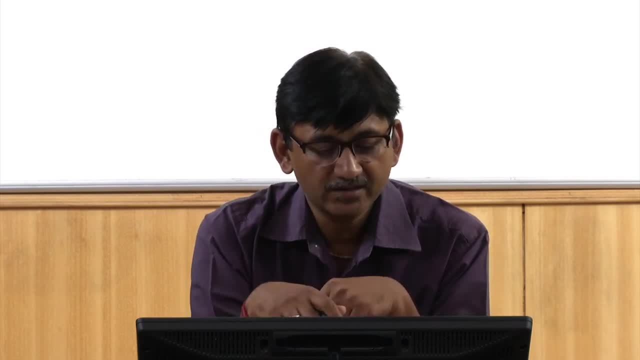 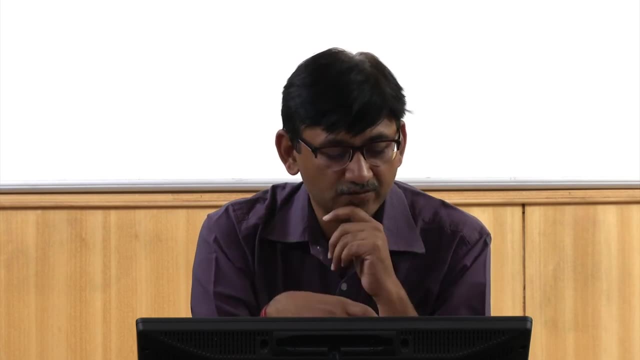 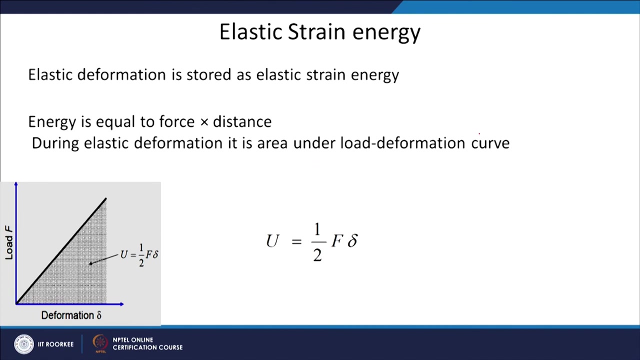 under elastic limit. So elastic deformation is stored as elastic strain energy in the material. and how? what do we mean by energy? It is equal to force into distance. So during elastic deformation it is area under the load deformation curve. So if I, instead of plotting stress versus strain, if I plot deformation versus load area, 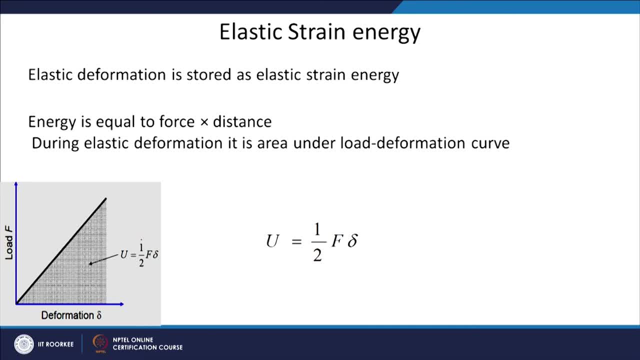 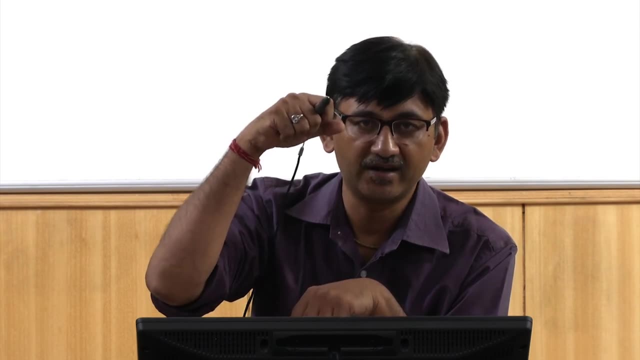 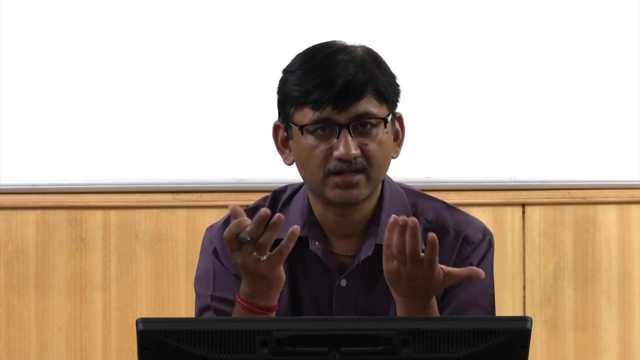 under the curve and area under the curve will be equal to half of force into displacement and that will give me the area under the curve. So this is my elastic strain energy which is stored in the material when I am deforming it. So when I release the force, this strain energy will be recovered and, of course, this energy